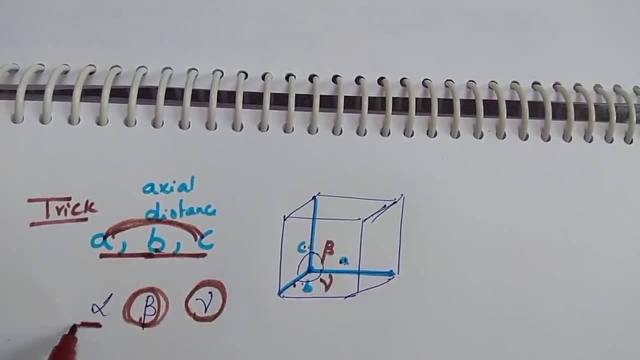 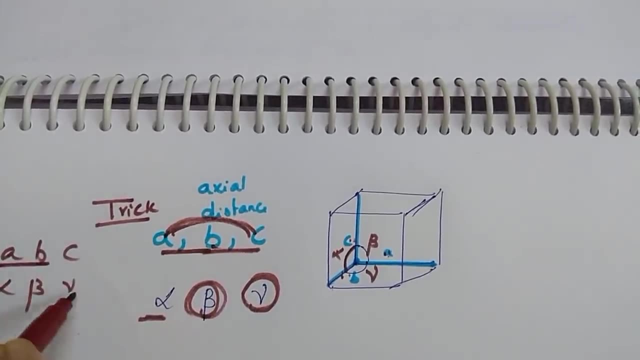 between A and B, what is the angle you need to take beta, and between A and B, what is the b and c, b and c, what you should take? alpha so alpha. so a, b, c, alpha, beta, gamma. between these two, the angle should be this one. you should not take these two. okay, between a, b, the angle will. 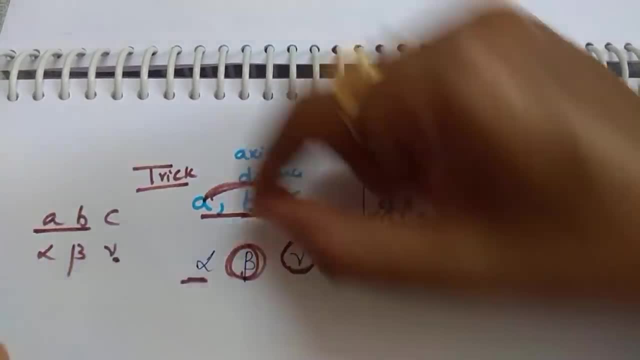 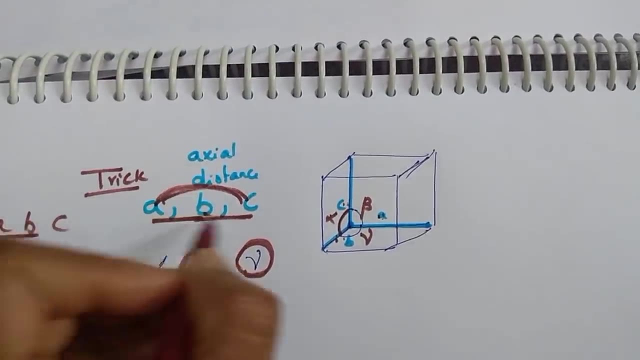 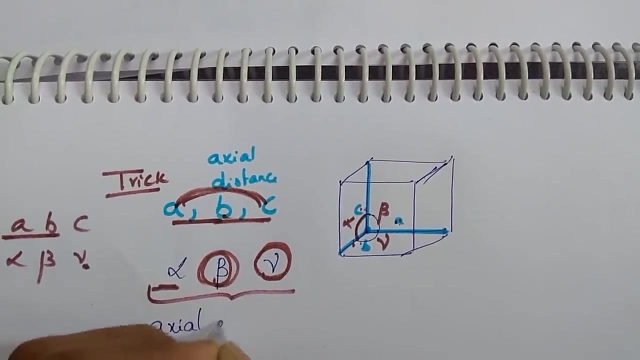 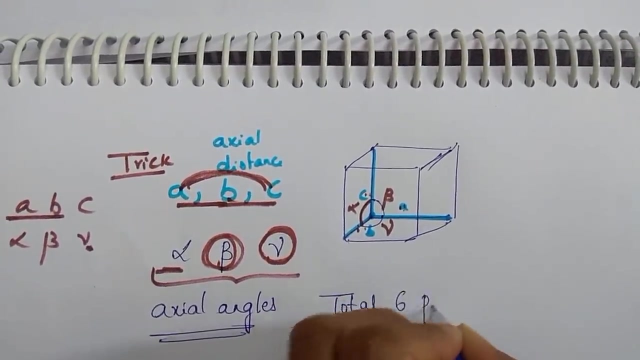 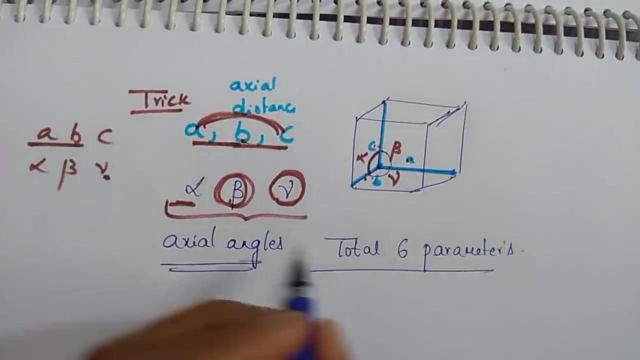 be gamma between b- c. the angle would be alpha. between a and c, the angle will be middle, one, clear. and here total. how many? three axial distances and three axial axial angles, axial angles, total, total. six parameters are required. six parameters are required to explain a particular unit, cell. six parameters we want. what are those six parameter? students a, b, c. 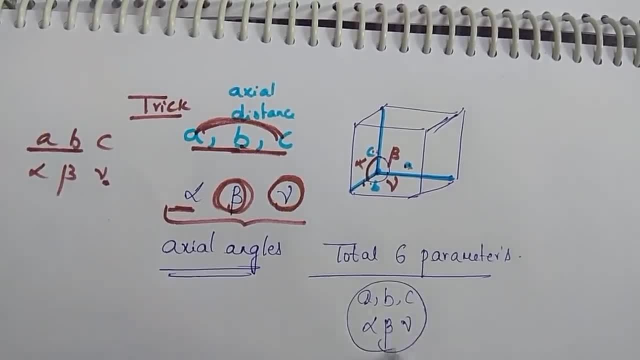 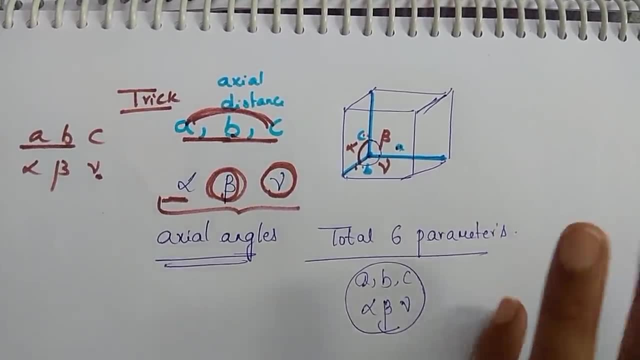 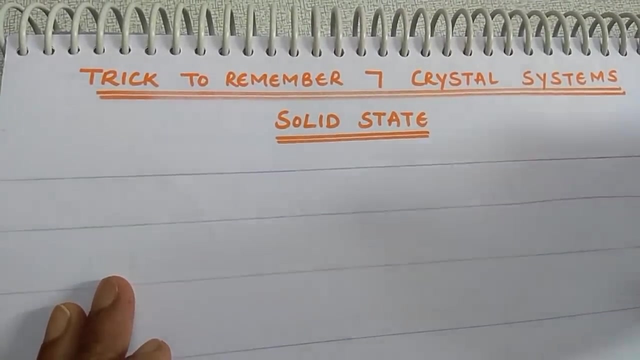 and alpha, beta, gamma. based on these values, the crystal systems, these unit cells are of, you can say, seven crystal systems. what are those seven crystal systems? those seven crystal systems are: cubic crystal system, tetragonal crystal system, orthorhombic system like this. seven systems are there actually? 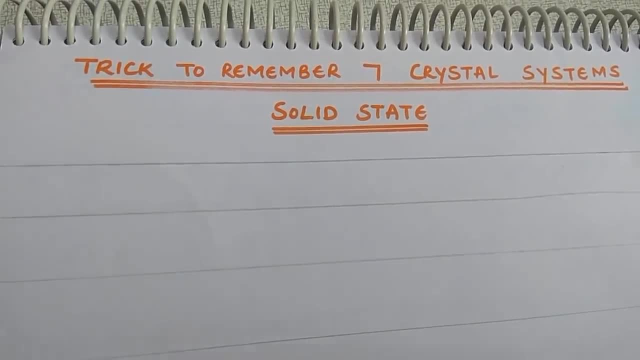 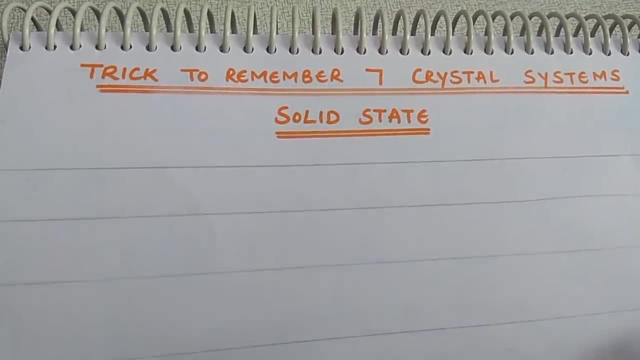 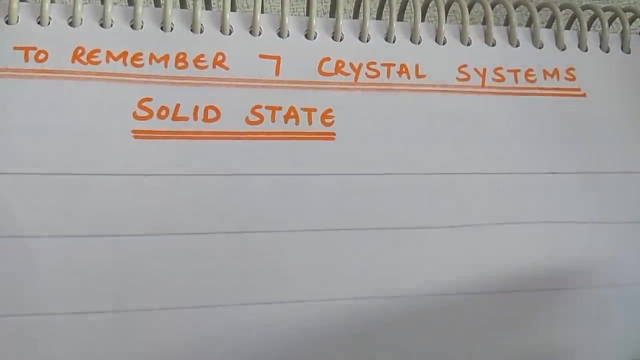 but if you observe your ncrt textbook or your college material or school classwork, you may feel difficulty to remember all those seven crystal systems. this video clears your concept and makes this concept easier. now i will tell you a small trick. okay, remember that, then your job will be easy. 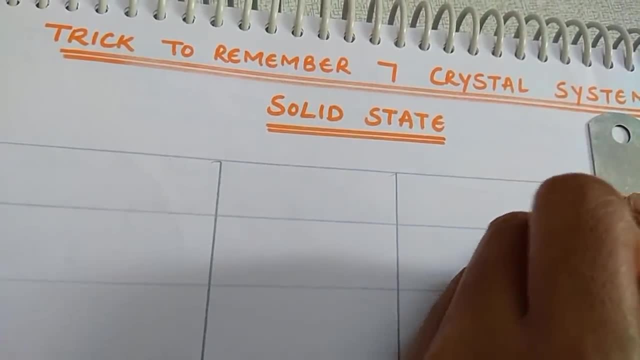 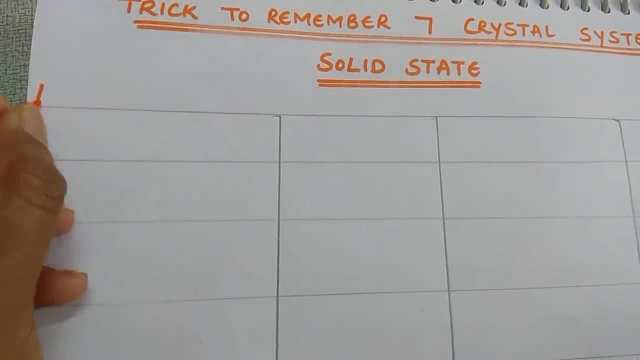 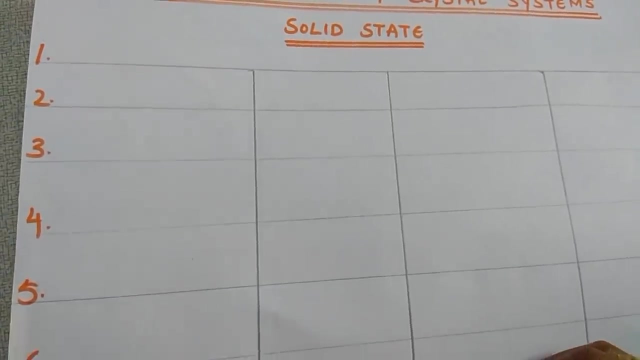 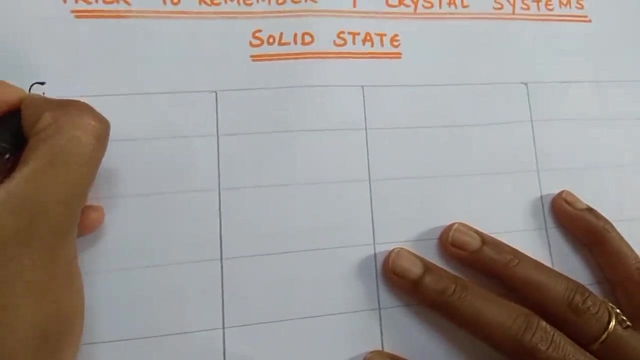 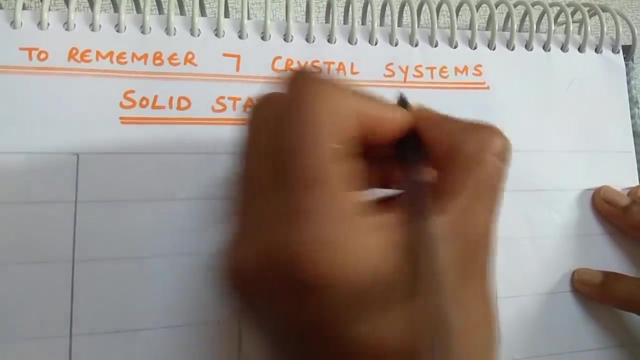 total, how many crystal systems? students, seven crystal systems. so name seven, one, two, three, six, three, four, four, five, six, five, six, oh, seven, one box, fine, now first one, see tricky CT HD, OMT. what is the trick? trick I'm reading here, trick is CT HD o t, HMT. 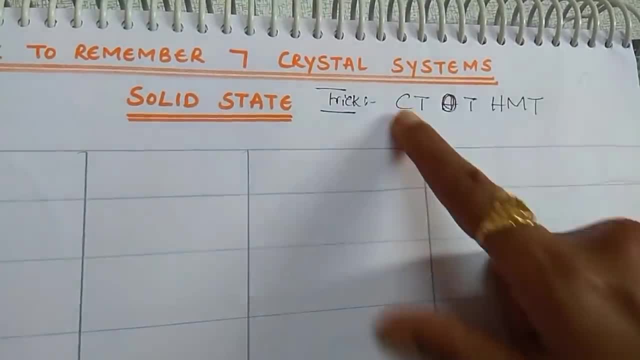 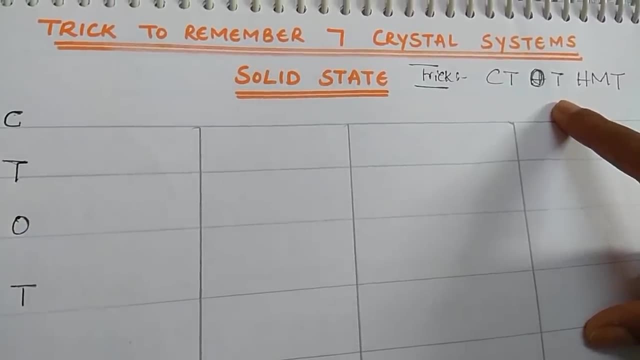 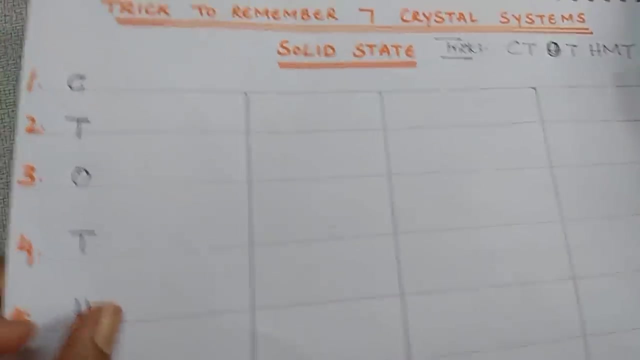 oh sorry, O T HMT. what is the trick? CT或 O T HMT. CT O T HMT. ok, CTivia electric Felliano. now this is for CMT. O T H M T. This is the trick. C T O T H M T. You have to remember like that. 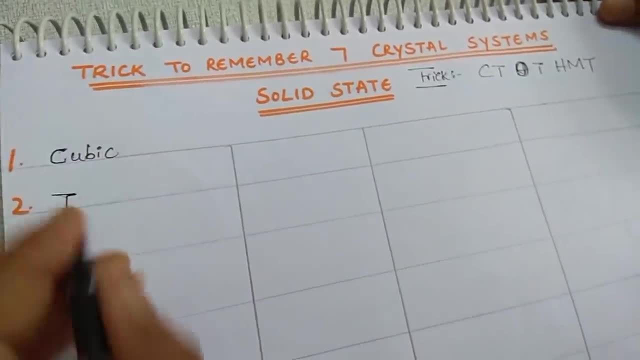 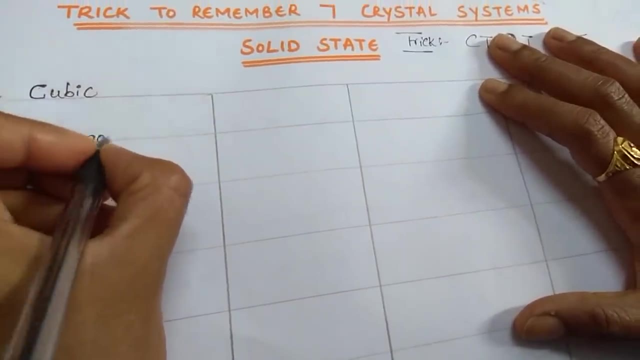 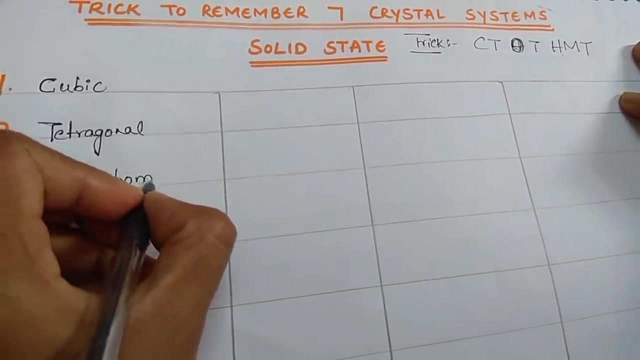 C stands for cubic. What C stands for Cubic And T stands for tetragonal. What T stands for students, Tetragonal. O stands for orthorhombic. O stands for orthorhombic And T stands for. 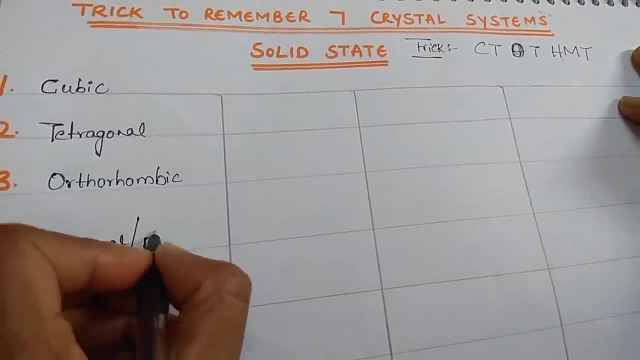 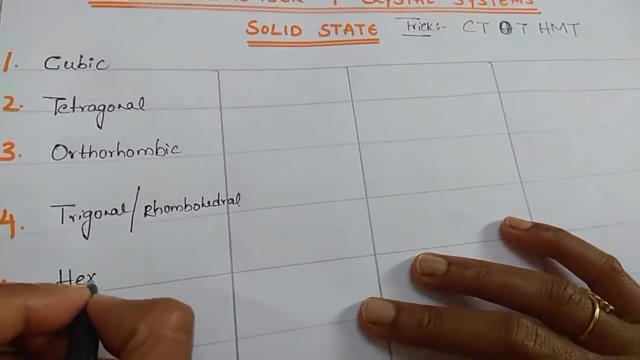 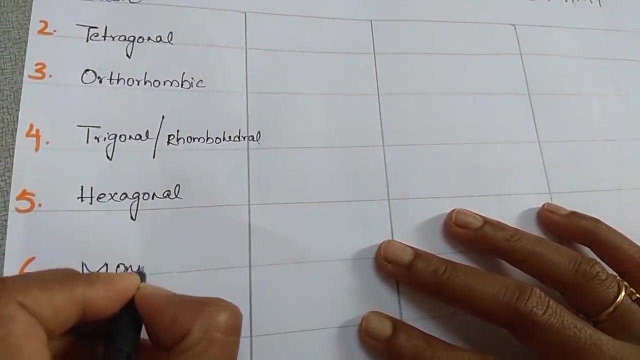 trigonal, or which is also known as rhombohedral. What is this, Which is also known as rhombohedral? And H stands for hexagonal. What is a H here? Hexagonal? What is M? M is monoclinic. What is M? 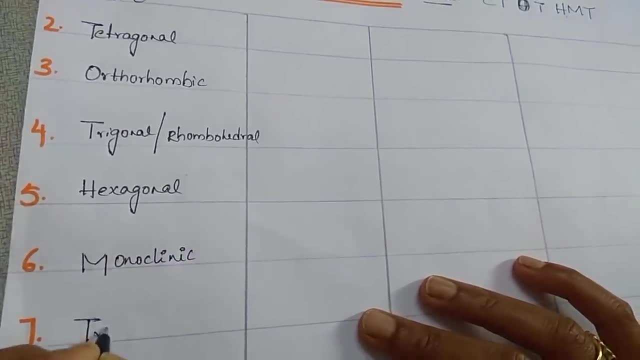 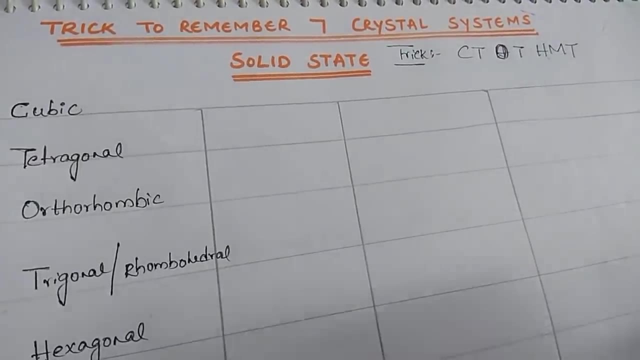 here Monoclinic, Monoclinic. What is T here? Triclinic, Triclinic. See, these are the seven crystal systems. Okay, But how? you have to remember C, T, O, T, H, M, T, If you change the order based on your reference. 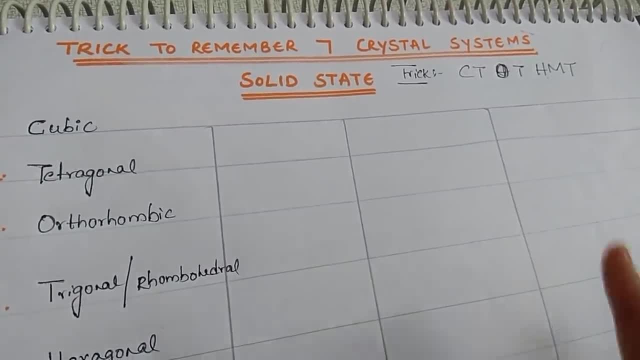 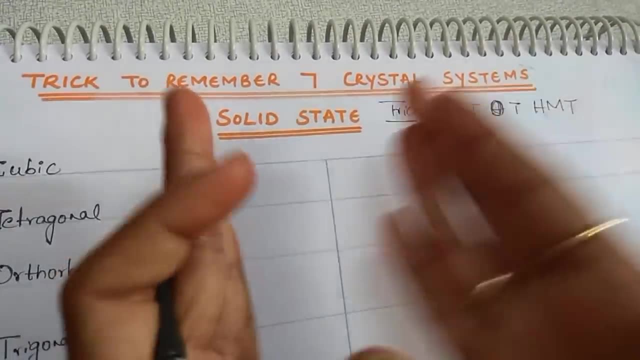 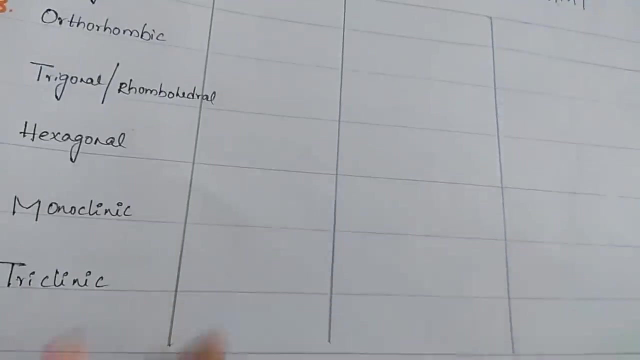 book, then you will get definitely confusion. If you want to score good marks from this chapter, this tabular column is most most important. Let us see the first column. I am writing for axial distances. Actually, I forgot to leave one box here, So the heading to this box I am keeping here, students. 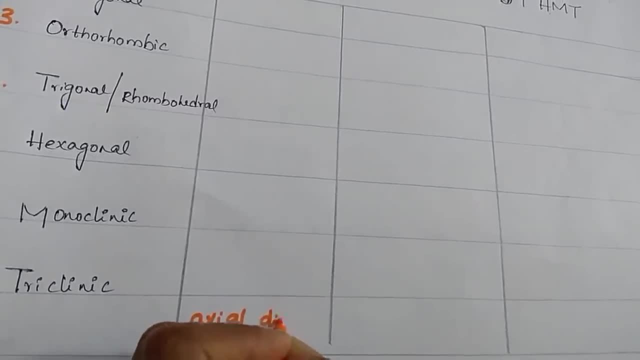 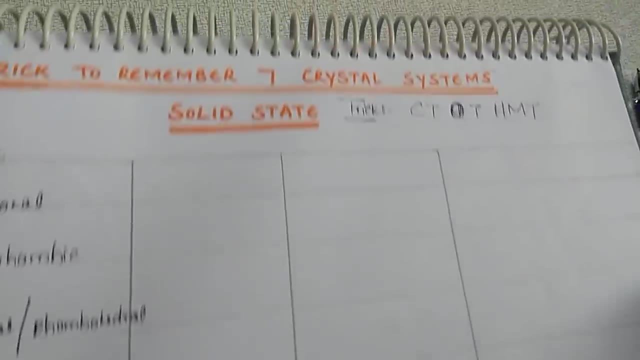 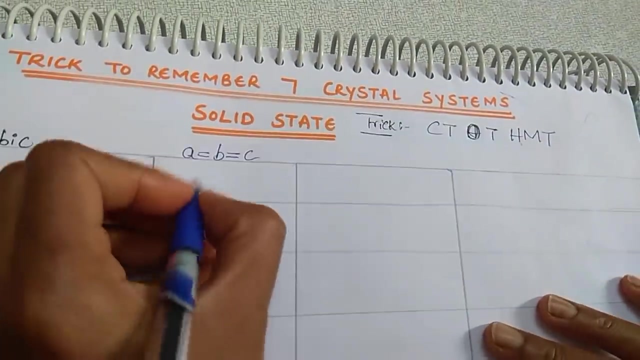 axial distances. This box is for axial distances. Okay, What is this? axial distances- A, B, C. See how I write, How easily you can remember. First, A is equal to B is equal to C. Okay, Next A is: 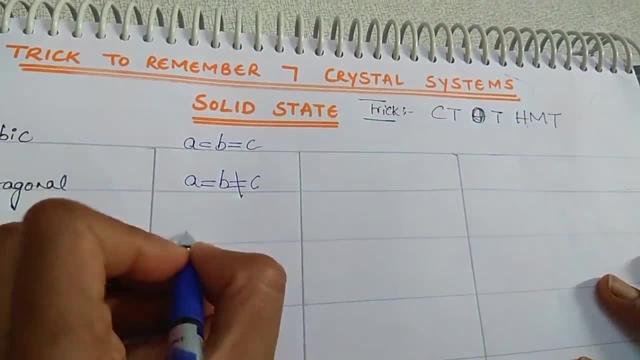 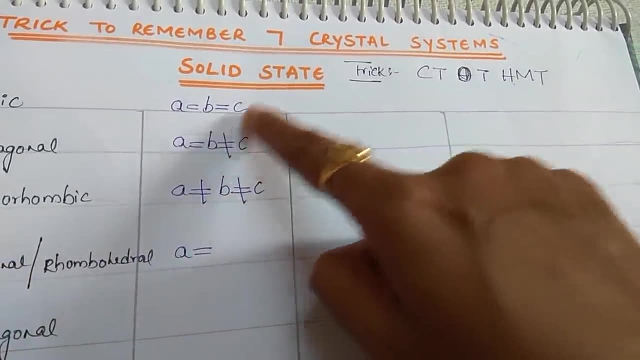 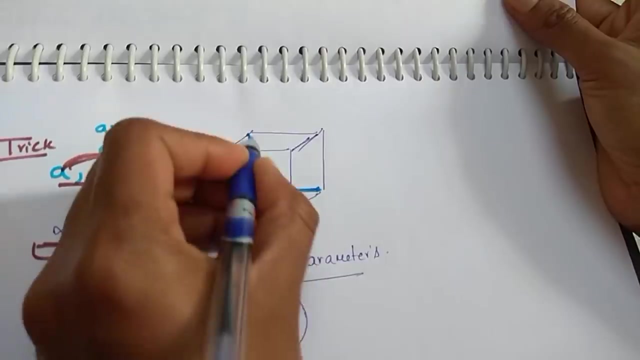 equal to B, which is not equal to C. Next one is: A is not equal to B, This is not equal to C. And next again see: A is equal to B is equal to C, which means that all the angles are same Here. all the distances are same: A length, B length, B length and C length, All the 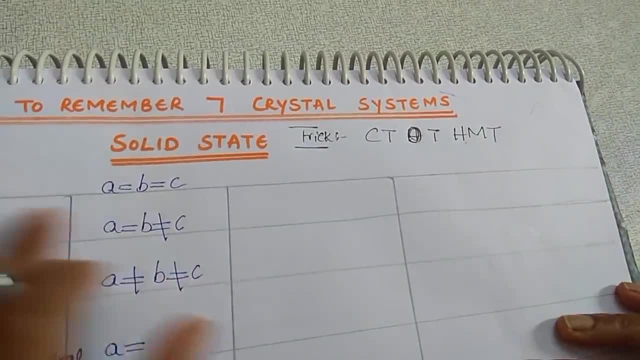 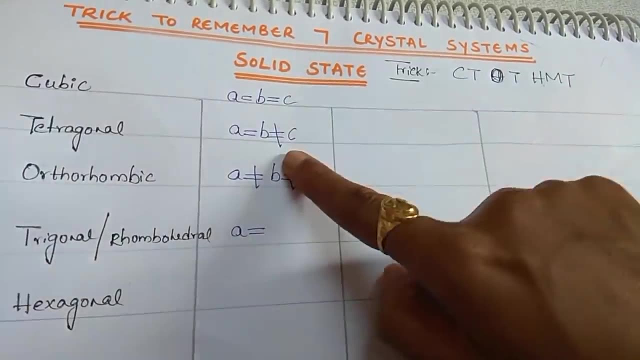 lengths are same And we call that as an cubic. here Cubic A, B, C are same. I will discuss about this. also, A is equal to B, is equal to C, And here A is equal to B, which is not equal to C, But in 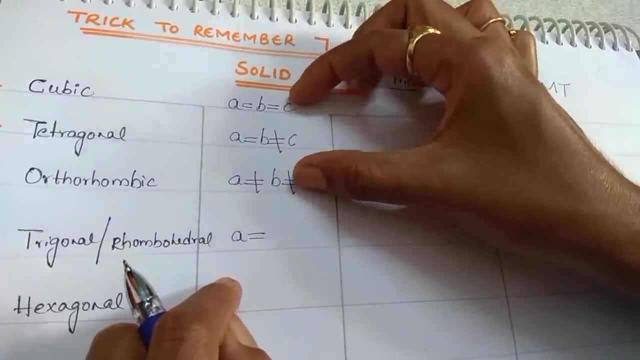 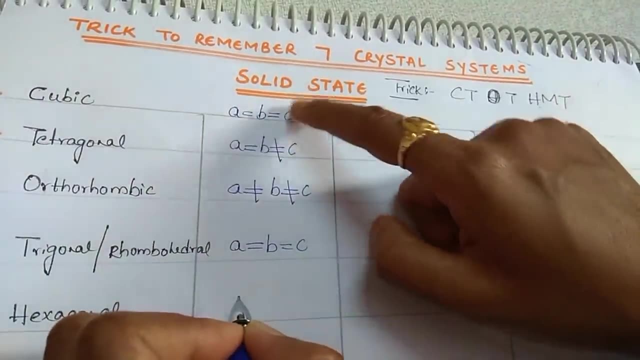 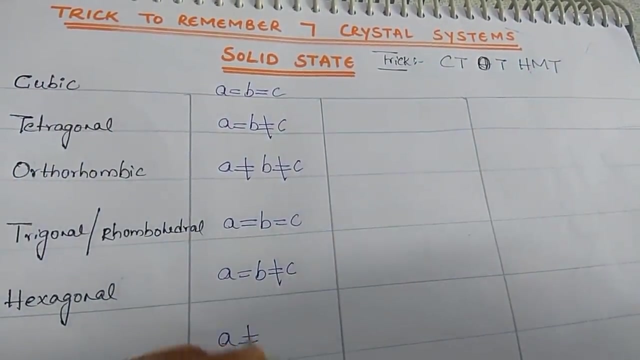 cubic three are not equal. Once you write up to here again, you have to repeat Clear students again you have to repeat. That is the easiest way. Again, repeat: A is equal to B is equal to C. Next, what will come? A is equal to B, not equal to C. What next way it will come? A is not equal to B is. 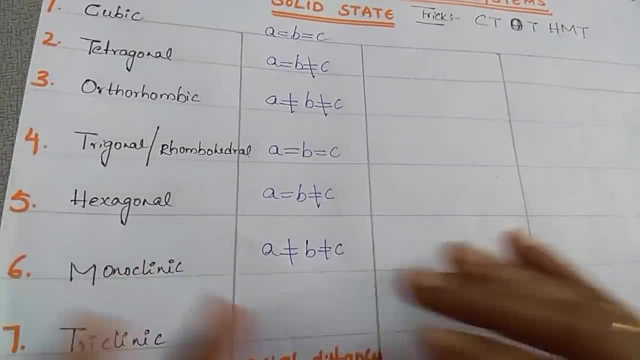 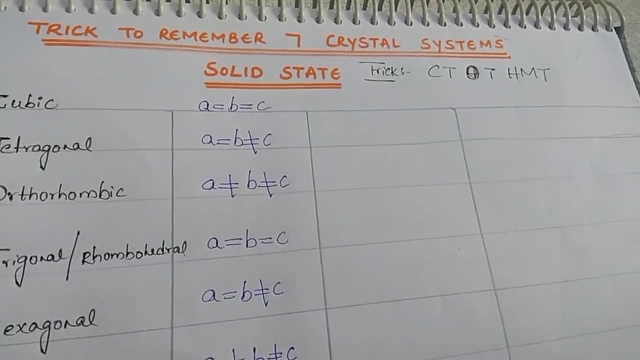 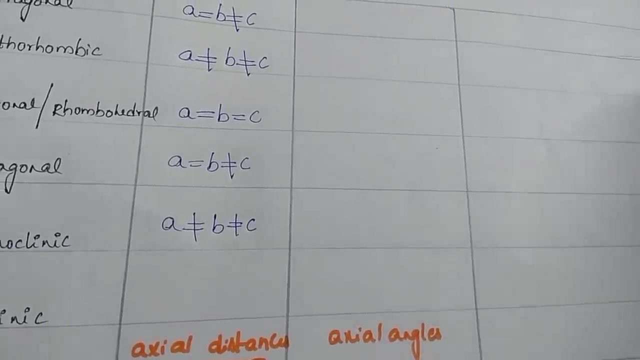 not equal to C. Okay, Coming to the last one. this one I will discuss with you, Wait. And coming to the next one: axial angles Here, what is that? Axial angles? What are these axial angles? Alpha beta and gamma Alpha beta. 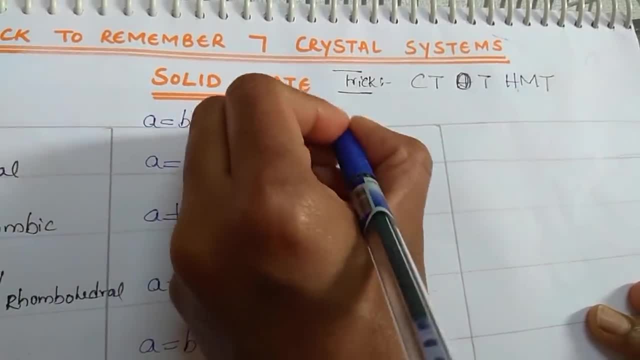 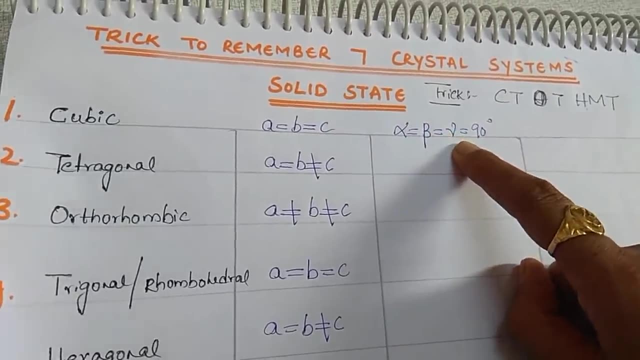 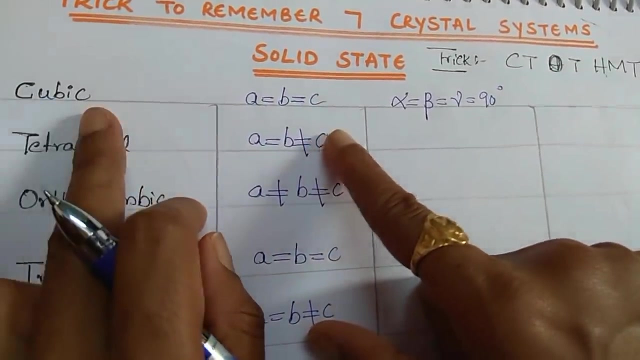 gamma. Alpha, which is equal to beta, is equal to gamma, equal to 90 degree. in case of what? In case of cubic system, alpha, equal to beta, equal to gamma, is equal to 90 degree. Clear, Clear. So observe here: in case of cubic system, A, B, C are equal. 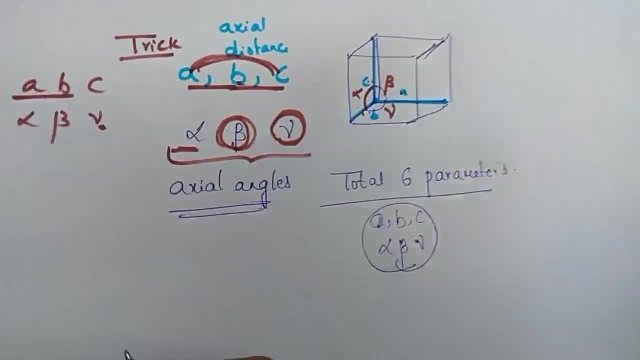 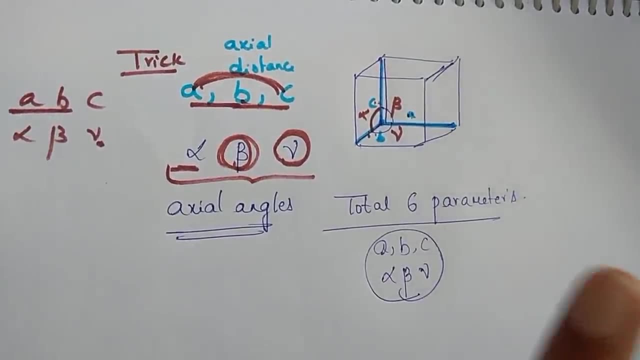 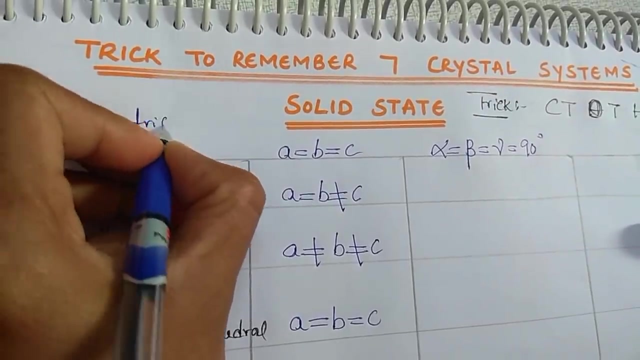 A, B, C are equal And alpha, beta, gamma also same, 90 degree only. So the system in which even axial angles and axial distances are equal, then that system is a symmetrical system. This is the most important objective question. Which is an symmetrical system? Which system is symmetrical? 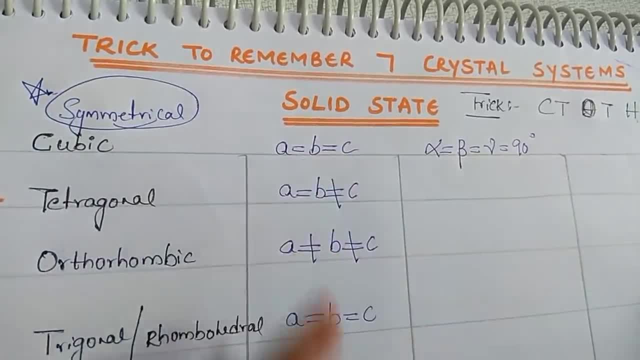 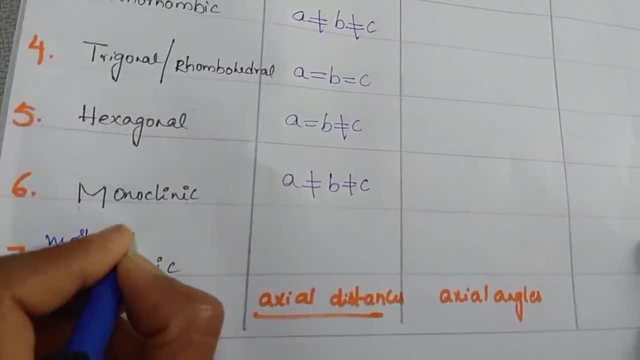 Cubic system is symmetrical. So this one is a symmetrical And the most unsymmetrical system- most unsymmetrical system is Unsymmetrical system- is triclinic system. See students here. this is a more unsymmetrical system. 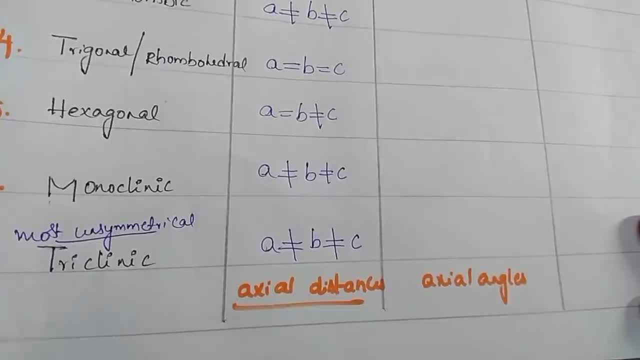 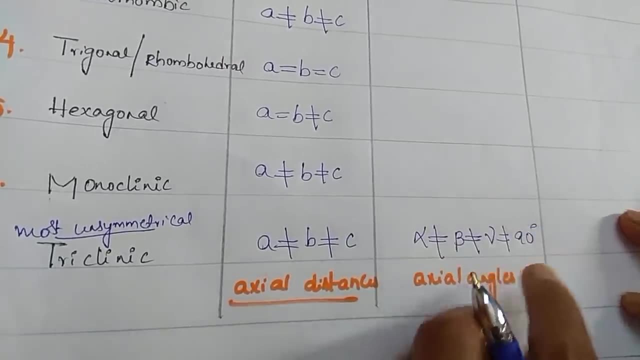 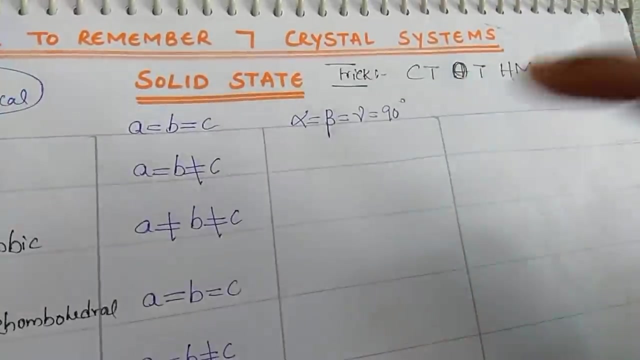 where A is not equal to B, is not equal to C, And whereas alpha is not equal to beta, is not equal to gamma, is not equal to 90 degree. This three are also not equal. This is also not equal. That system is a triclinic system. This is an important one. And how can you remember this part, This part? Okay, 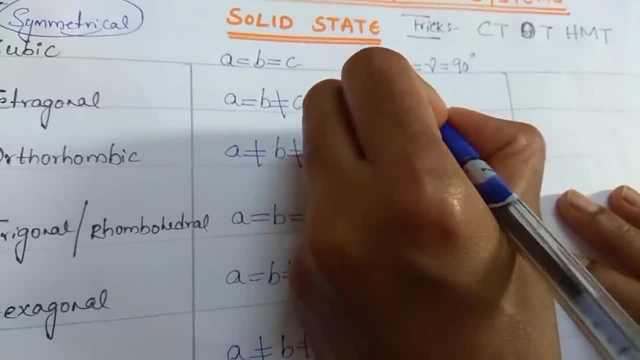 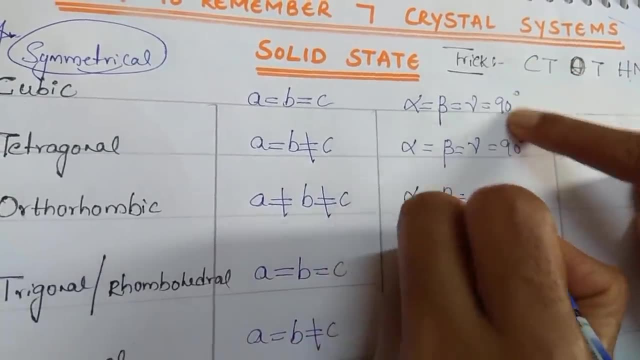 In case of tetragonal alpha, equal to beta, equal to gamma, is equal to 90 degree, And here this is also same. First three are same. Clear First three are same, No confusion. And last one is not equal to So. 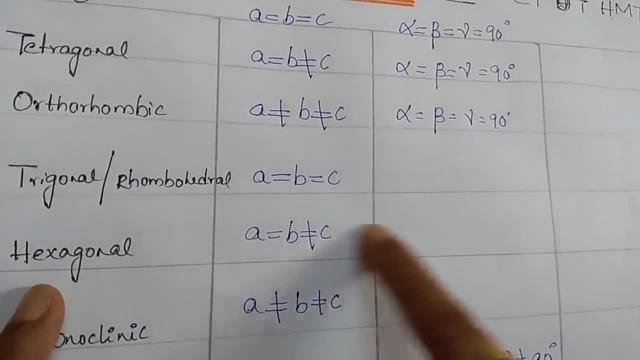 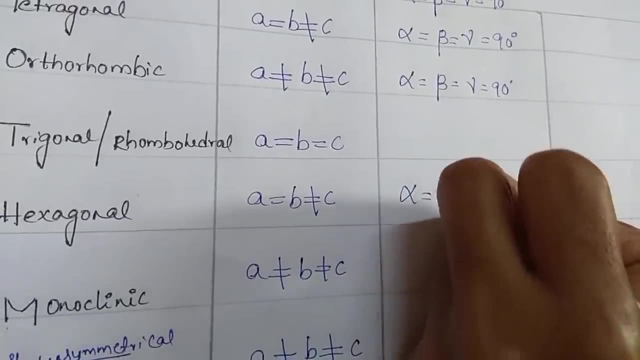 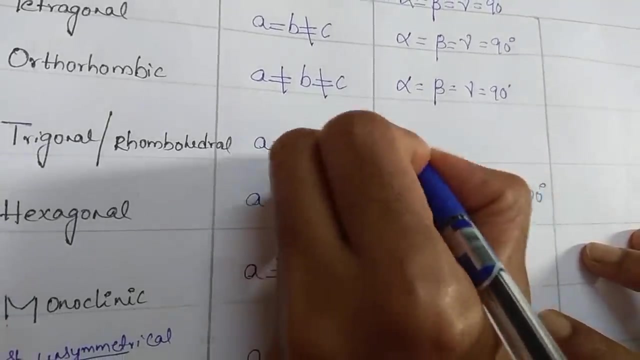 no confusion. Now coming to the hexagonal part. Next, you should remember this part to avoid confusion: Alpha beta equal to 90 degree, Whereas gamma equal to 120 degrees in this case. Okay, fine, Easy. After that, this part: if you see alpha beta, gamma which is not equal to 90 degree, 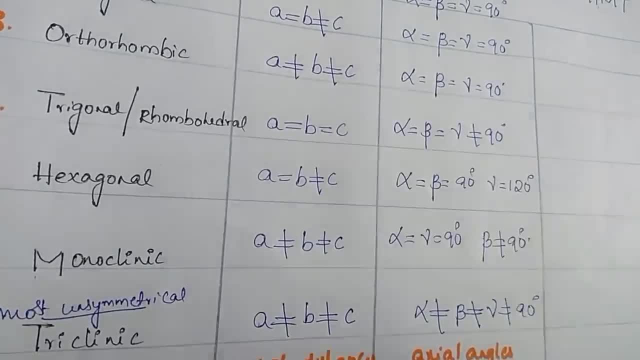 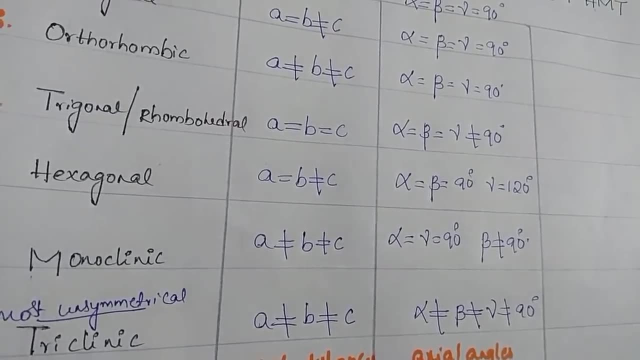 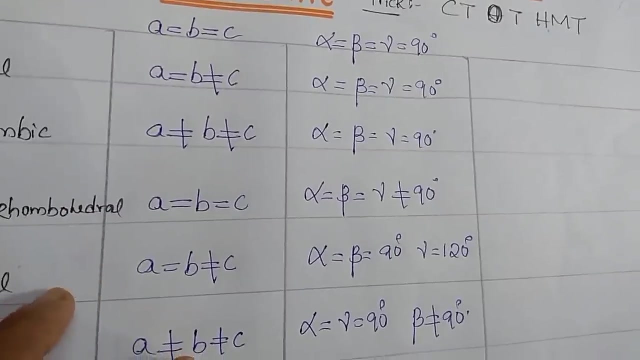 Hexagonal. you write. After that these two you should write. Then only you won't feel confusion. And from this they are asking the questions in an objective examination Like NEET, JEE SET. these are the most important questions. And one more thing: examples. It is important, It is. 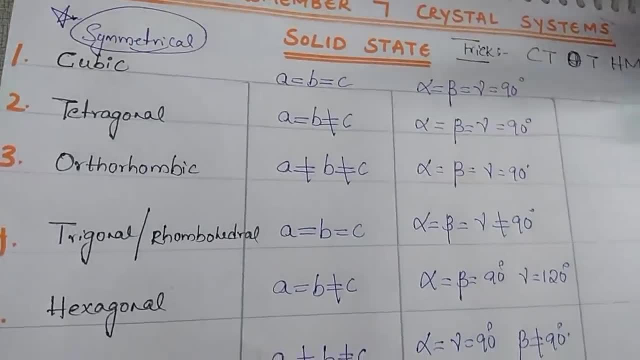 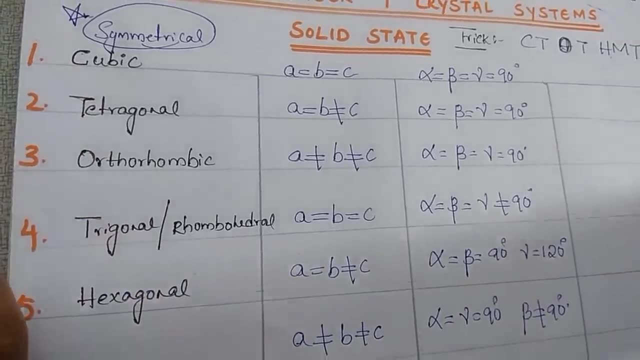 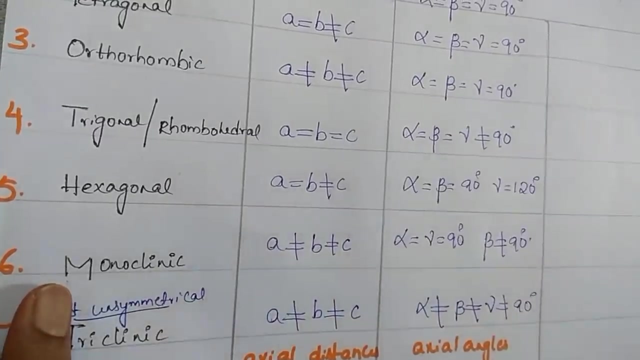 important to. Next important part is examples, Examples. you need to concentrate How many examples you can remember for each crystal system. it completely depends on your memory. I will give you most important examples, but practice students three to four times. This is because this is the most important. 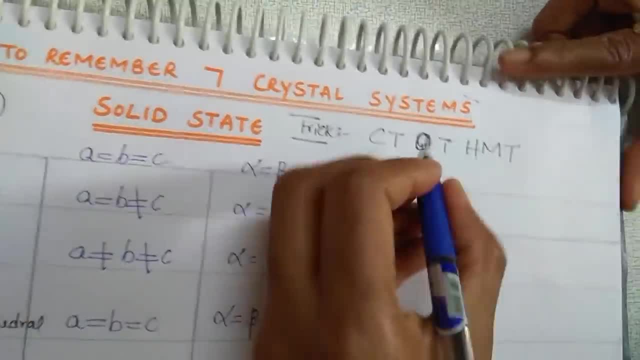 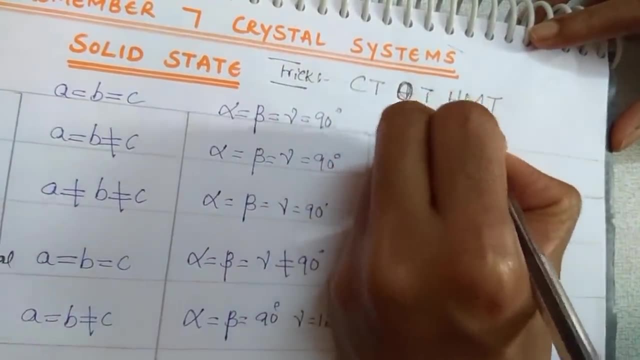 part. Cubic system. Cubic system Examples are NACL- I will use black pen- NACL, KCL And you know zinc blend. Zinc blend means Z and S is a zinc blend And you can see copper. 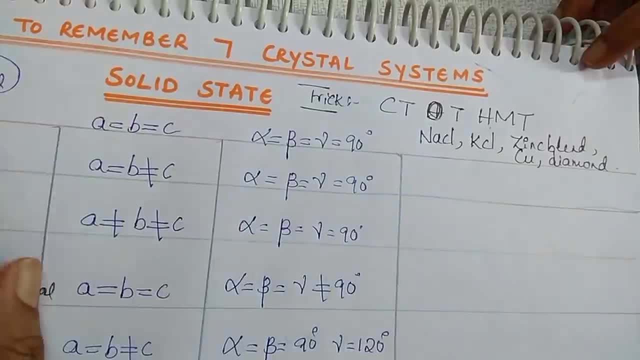 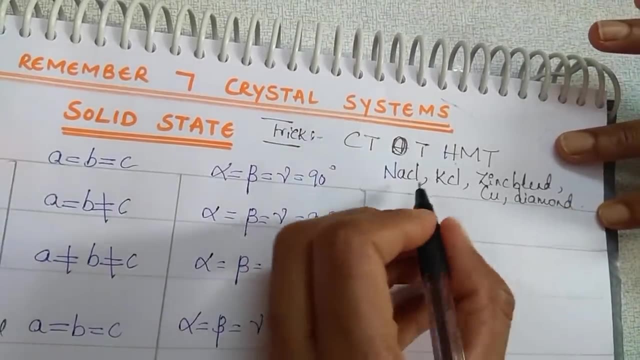 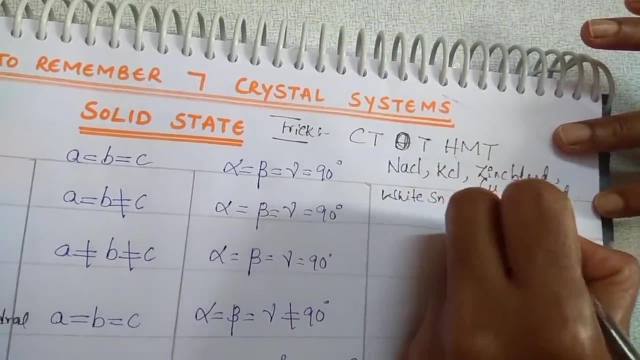 diamond are the examples for what you know cubic system. They will ask you an exam. Next one is tetragonal system. In case of tetragonal- you can see the examples- are like white tin. white tin, SNO2, TiO2 and calcium sulfate. These are the examples for tetragonal. 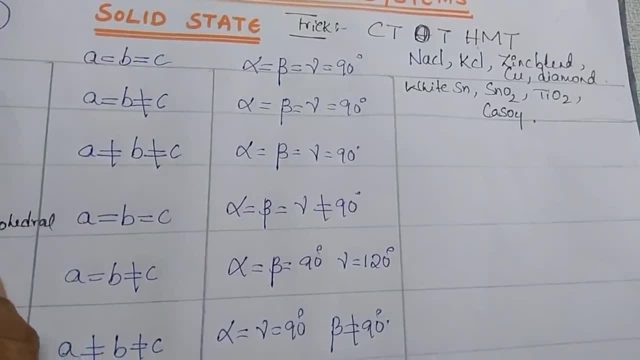 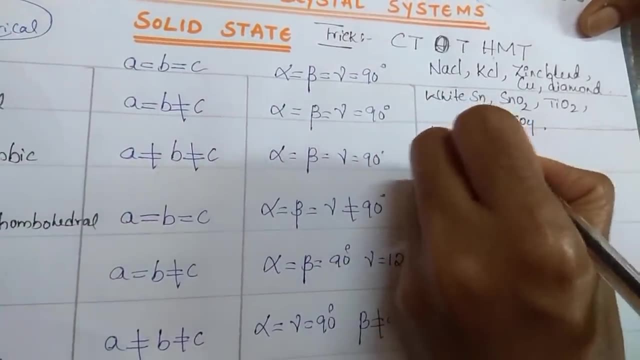 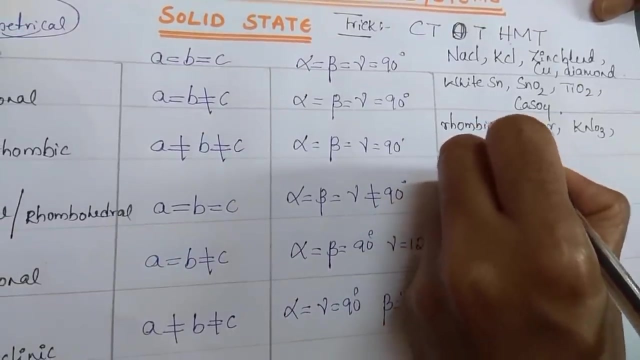 system. Okay, And and next one is orthorhombic system. In case of orthorhombic system, examples are rhombic sulfur, rhombic sulfur KNO3 and BS44.. These are the examples You can take. 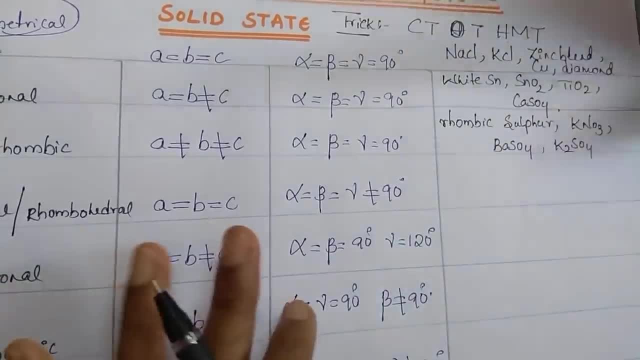 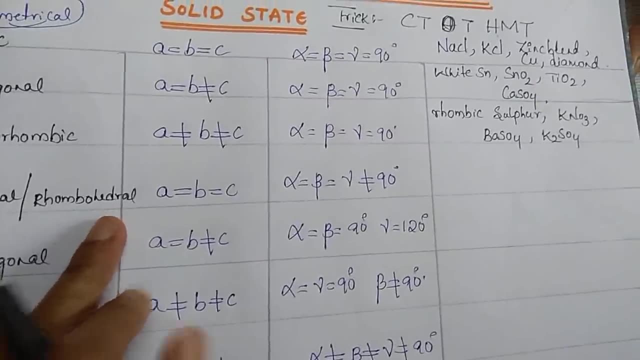 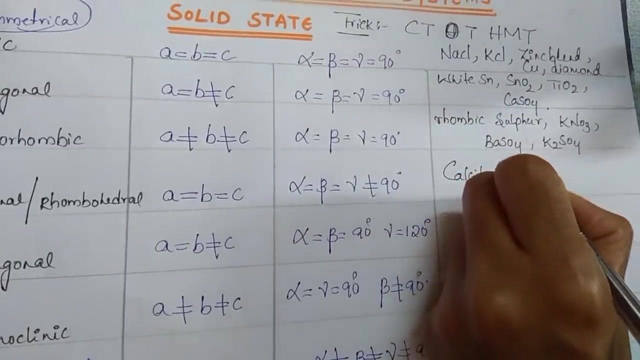 K to S44. also, How many examples you can remember, that is up to your memory, but it is important. Coming to the trigonal or rhombohedral, The examples for this Next one is calcite and ginsite. Calcite is a calcium carbonate and you can say cinnabar.